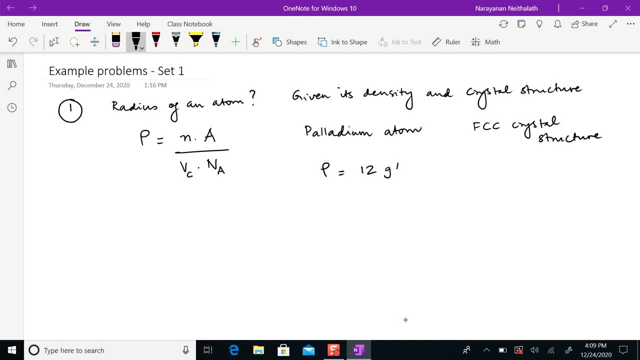 palladium is given as 12 grams per centimeter cube. So you're asked to find the radius of this atom. So we're going to use this equation: Rho is N times 8 divided by VCO times NA, And since it's an FCC crystal, you now know that the value of N is 4.. 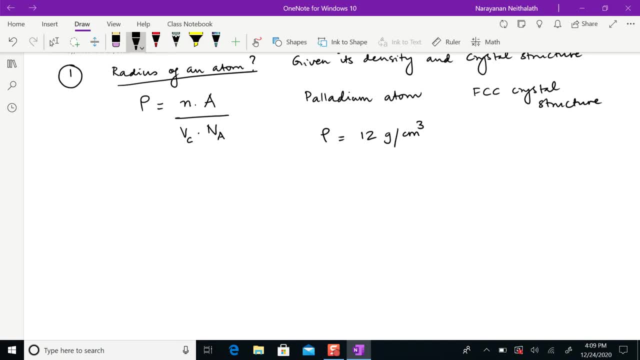 There are 4 atoms per unit cell in an FCC crystal structure. Therefore we're going to say 12 grams per centimeter cube. Be very careful with the units Gram and centimeter. cube is equal to 4, number of atoms in the unit cell. 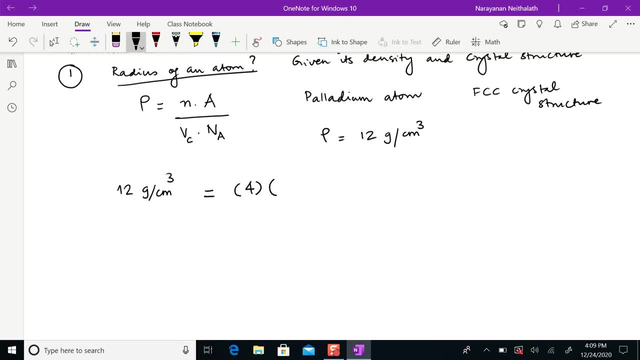 and then atomic mass of palladium. You can look at the periodic table. If not, it will be given. you can find it out as 106.4 grams per mole. That is the atomic mass of palladium divided by 106.4 grams per mole. 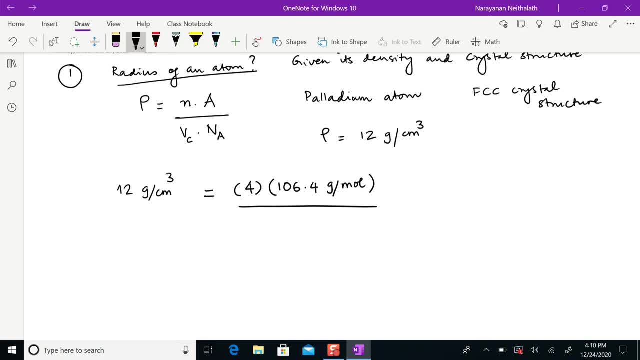 volume of unit cell. we don't know, and that's where we are going to get the radius from. so it's volume of unit cell times. avogadro's number is 6.023 times 10 to the 23 atoms per mole, right? so if you do this calculation, vc will then be 4 times 106.4, divided by 12 times 6.023 times. 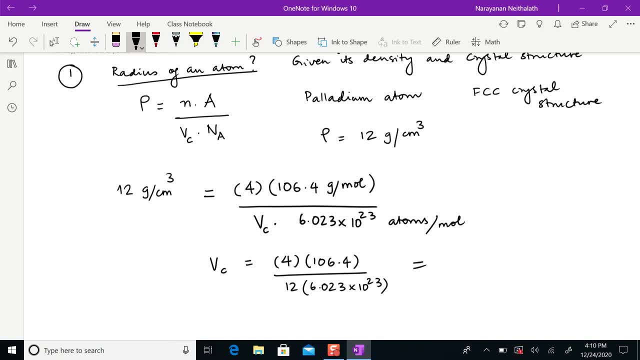 10 to the 23, you get volume of unit cell. you can do this calculation. you will get this as 5.88 times 10 to the minus 2. 23 centimeter cube. this is the volume of the unit cell. now, volume of the unit cell is equal to a. 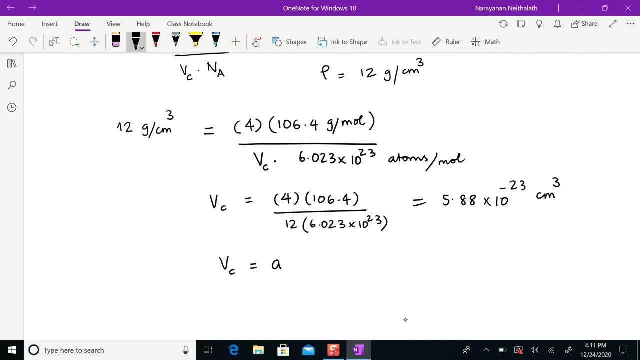 cube. so vc is equal to a cube, where a is a side length of the cube, which is equal to 5.88 times 10 to the minus 23 centimeter cube. from that we can find a, which is a side length of the cube 3.. 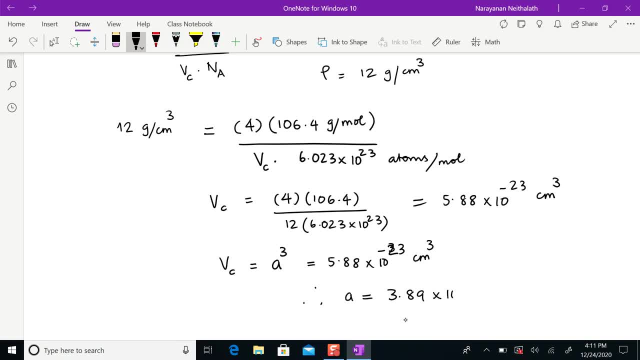 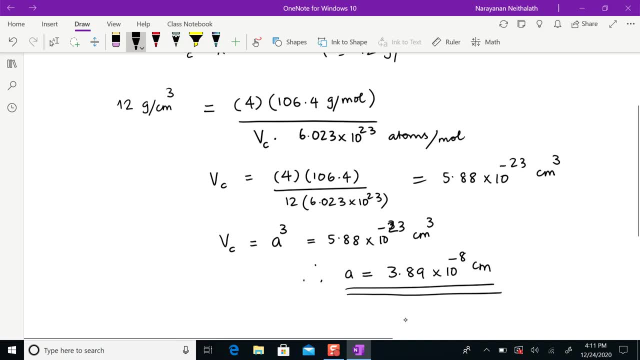 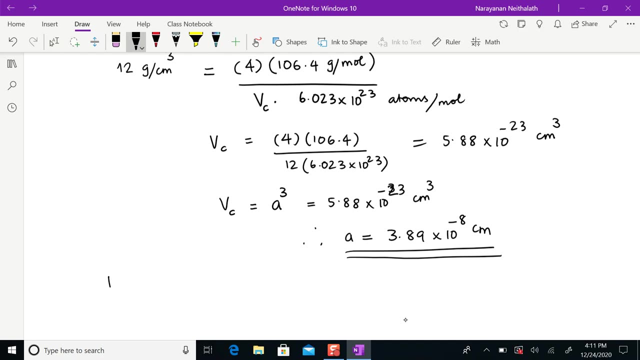 as 3.89 times 10 to the minus 8 centimeters. so you can do this calculation. you will get the side length of the cube as 3.89 times 10 to the minus 8 centimeter. now for an fcc unit structs. 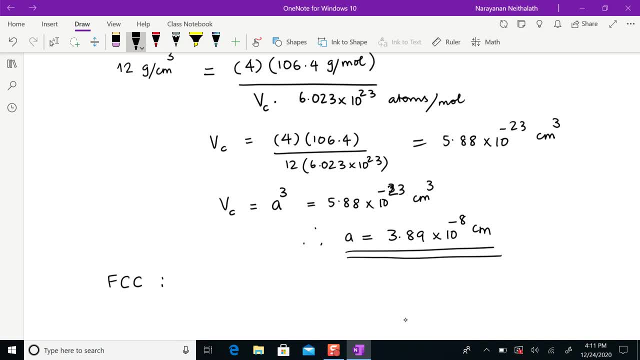 unit cell. you have seen that we have done the derivation. class 4r 4 times radius is equal to root 2 times a. therefore r is equal to root 2 times a over 4. you substitute this a here you will get r as 1.375 times 10 to the minus 8 centimeters. these are all atoms. they're very 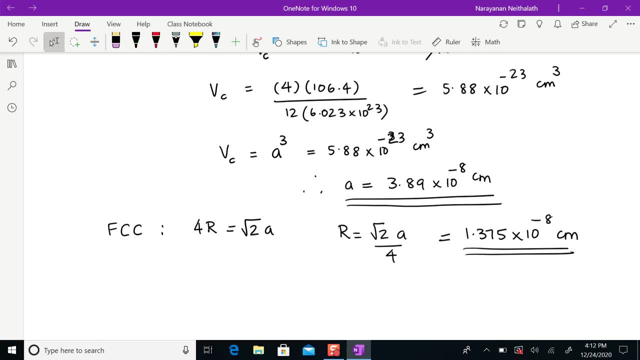 small, so we always use their radius in nanometers. one nanometer is 10 to the minus 9 meter, or you can do this as 0.1375 nanometers. this is the radius of the palladium atom and that is your answer. so you can do these kinds of problems, whether to find the radius or given the radius. 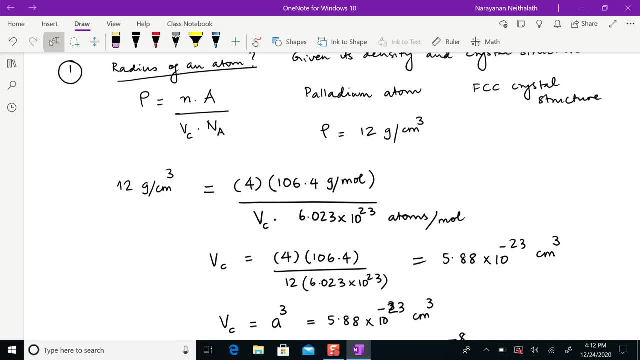 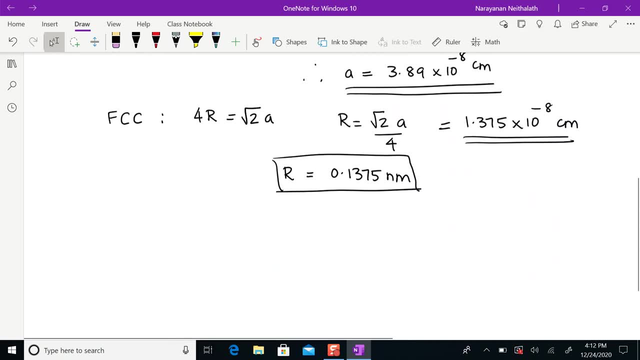 now, you can find the density given the radius, you can find what crystal structure it is and all of those kinds of problems. so this is one, one simple problem on crystal structure. now, the second problem that we are going to do today, which i'm going to show you today, the second type of problem is the one where we have the 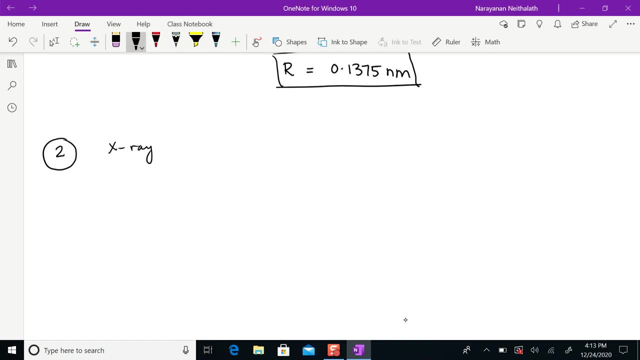 x-ray diffraction data- x-ray diffraction that we talked about in class to determine the crystal structure. so you have x-ray diffraction data. you know the wavelength of the x-rays- for example, lambda. so here i'm giving wavelength of x-rays as 0.1659 nanometers. so here is an x-ray with a wavelength of 0.1659 nanometers. 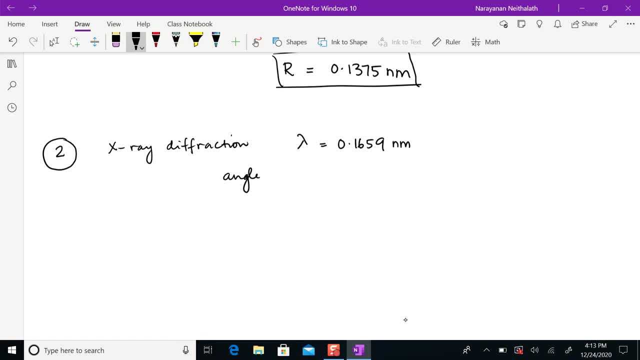 and the angle of diffraction. so this is diffracting on a crystal. the angle of diffraction is given as 75.99 degrees and you are having this diffract out of a c c crystal. you are asked to find out the lattice spacing the crystal lattice. 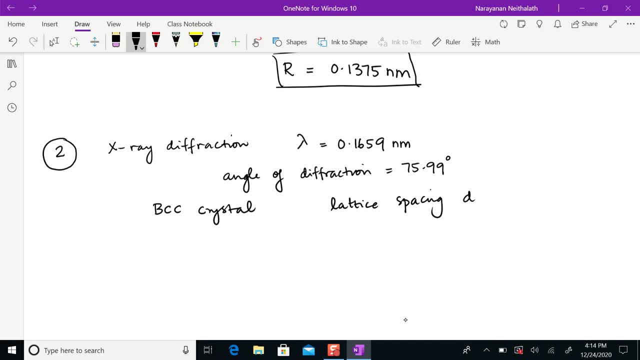 spacing D. that's a question. so you're going to basically make use of the equation n lambda is equal to 2d sine theta. this equation that you're going to use, angle of diffraction is given. know that angle of diffraction is equal to 2. 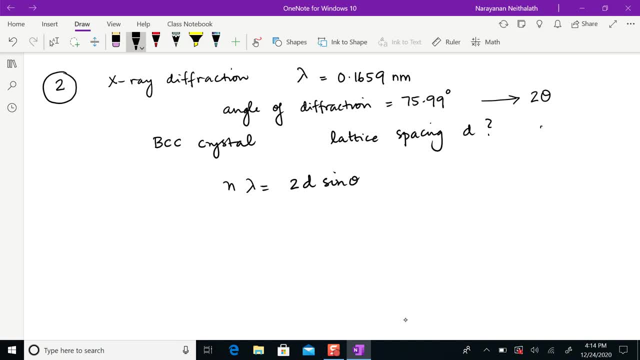 theta. therefore, theta is equal to 75.99 over 2 degrees n order of diffraction. if you are not given what the order of reflection is, you can take it as 1. so 1 times lambda 0.1659 nanometers is equal to 2d sine. theta is 75.99 over 2 when you're given the angle. 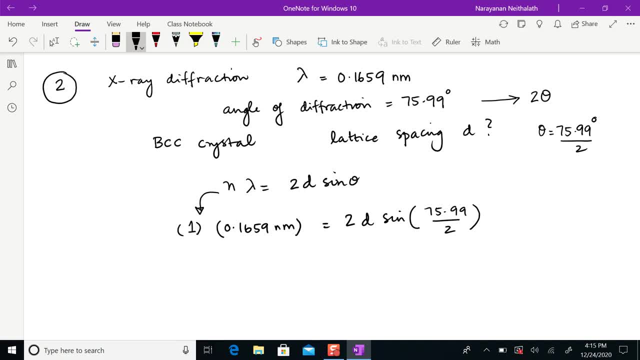 of diffraction. it always means 2 theta. so you have to divide it by half to get the, divided by 2 to get the value of theta. so from this you can get D as point 1, 3, 4, 7 nanometers. so this is the lattice spacing D. now, if you are also 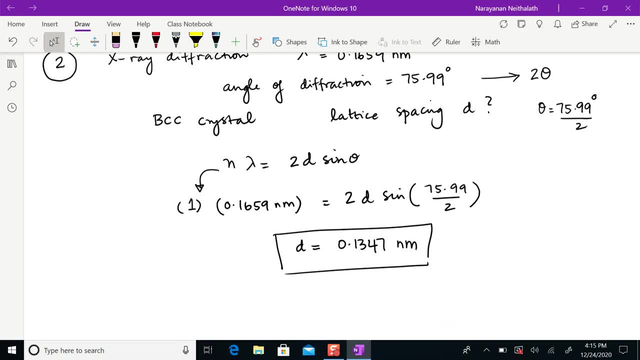 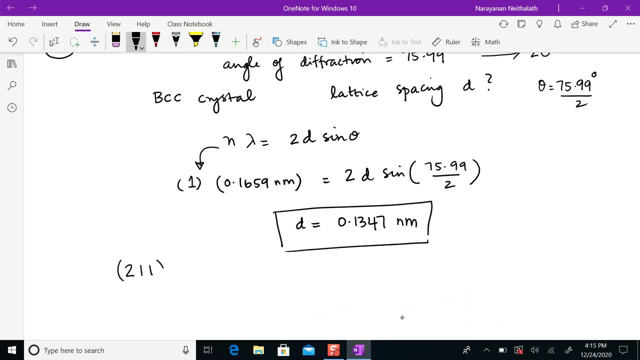 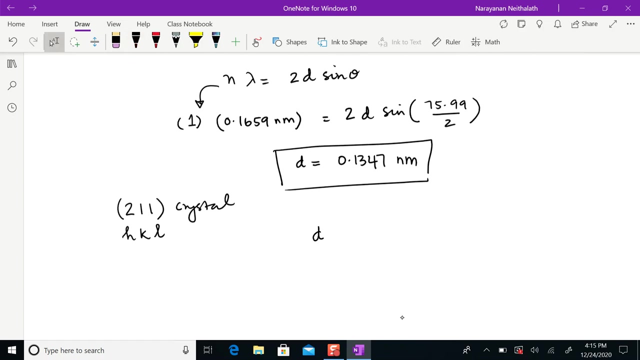 given that this is actually diffracting out of, say, a 2 1 1 crystal. 2 1 1 crystal- we have talked about this in class. 2 1 1 is basically the hkl indices of the crystal. so if this is a 2 1 1 crystal, you know that D is equal to a over square root of. 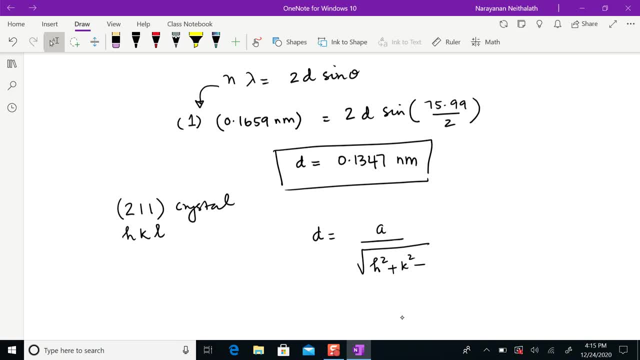 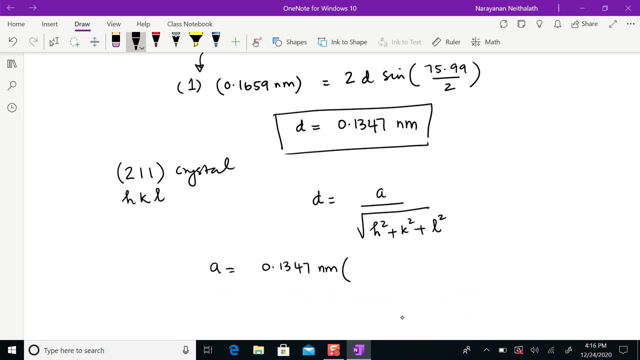 H square plus K square plus L square. so you know that. you know the value of D. you can find a as point 1, 3, 4, 7 nanometers times square root of 2 square plus one square plus one square, or you will get the value of a as point 3, 2, 99.